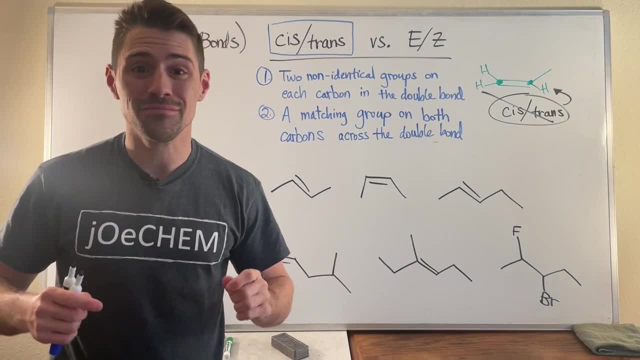 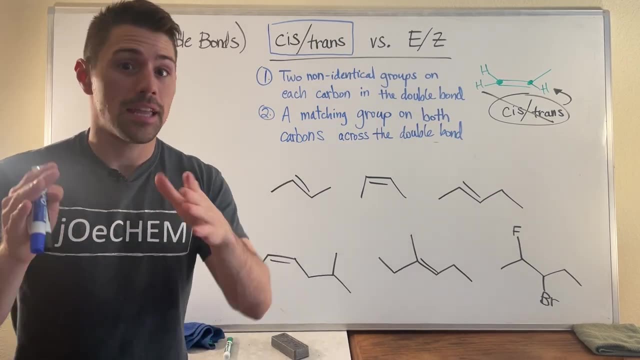 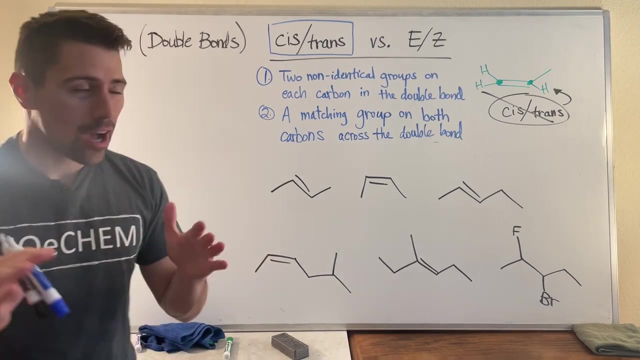 Hey gang and welcome back for another video here on JoChem Okay gang. so in this video I want to demystify a potentially confusing topic that I know was confusing for myself when I was taking organic chemistry, and that topic is when you're talking about double bonds. 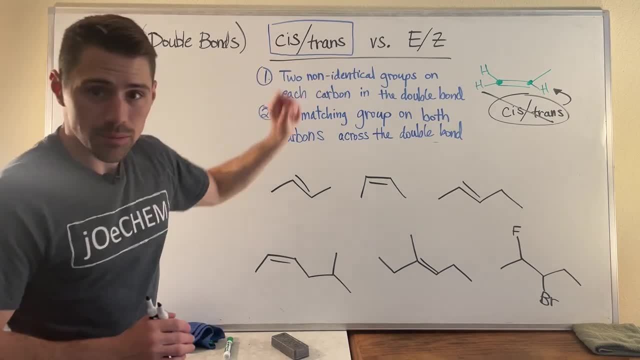 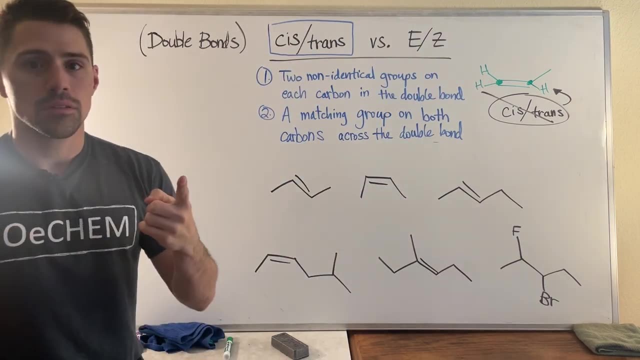 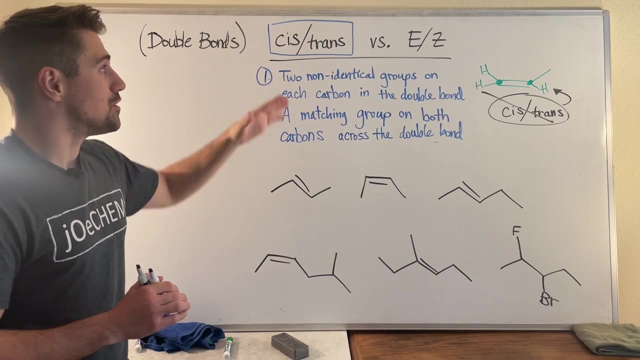 when you are able to identify if something is a cis-trans double bond or if you can't do that, can you label it as E or Z? So we'll go through what you need to evaluate to be able to call something a cis-trans double bond as well, as, if you can't do that, if you can call it an E and Z. 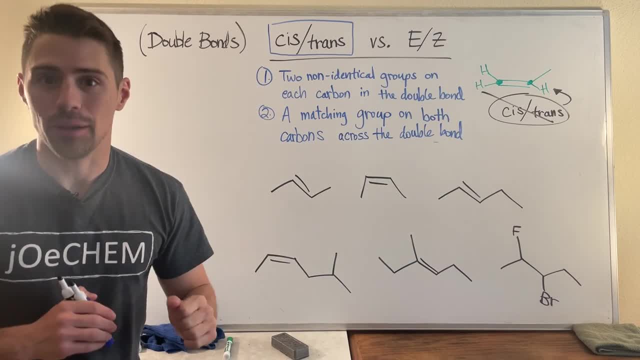 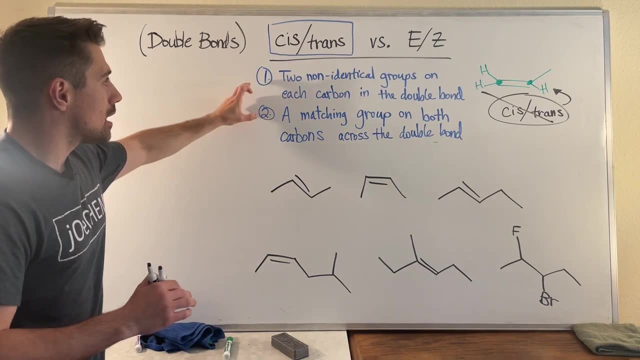 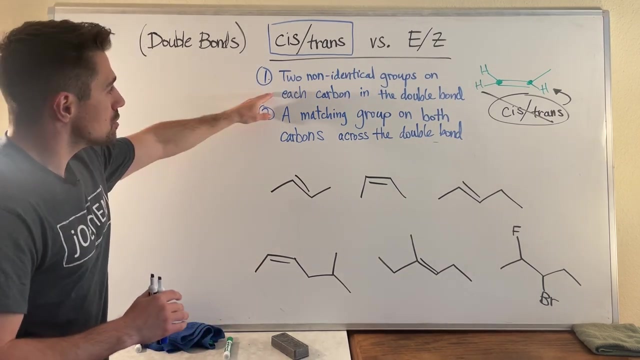 double bond, what E and Z means and how you go about doing that as well. So I want to start first with going the cis-trans route. So when you are looking at a double bond and figuring out whether it's cis or trans, you need to look at two things first. The first thing is is that when you look 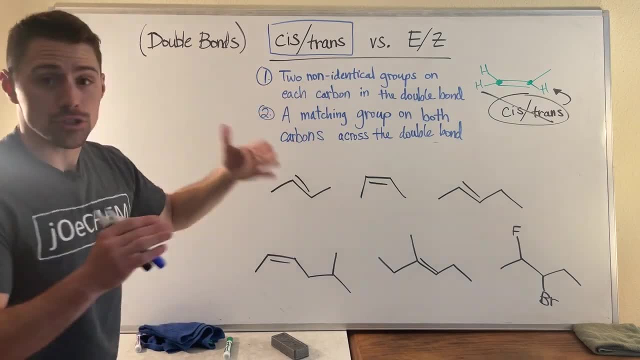 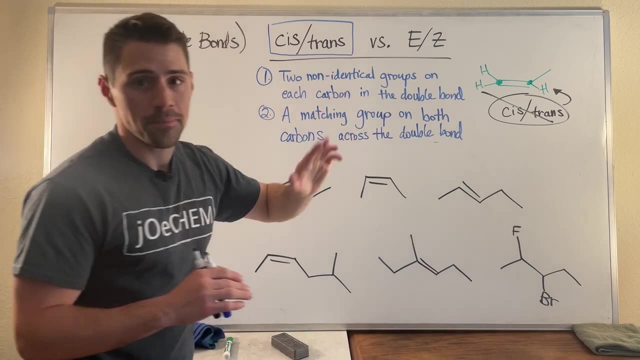 at each carbon in your double bond and you have to first check. okay, when I'm looking at each carbon, does each individual carbon in the double bond have two non-identical groups? What I mean by that is, if we look at this green structure over here, this is just a three carbon alkene. I kind 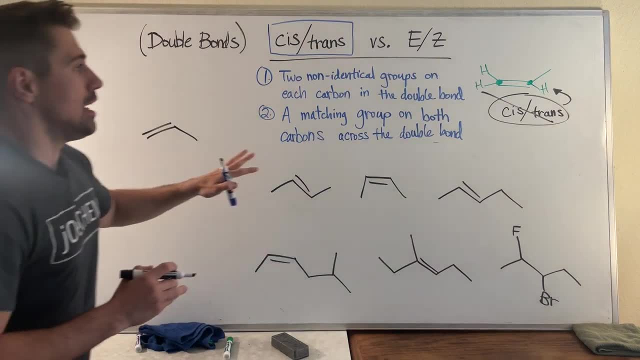 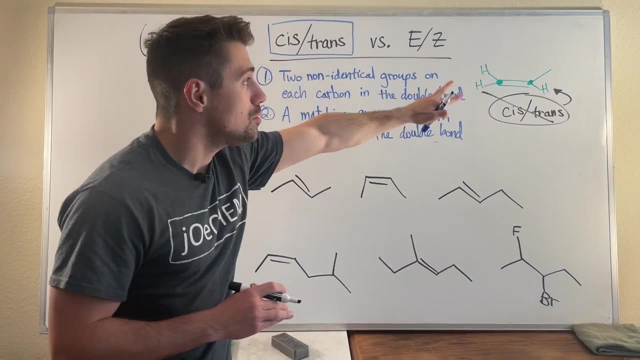 of drew it like upside down, but it looks like this If you look at both of these dotted carbons, the one on the right has a CH3 and a hydrogen, So those are two non-identical groups. That looks good for the first point we're. 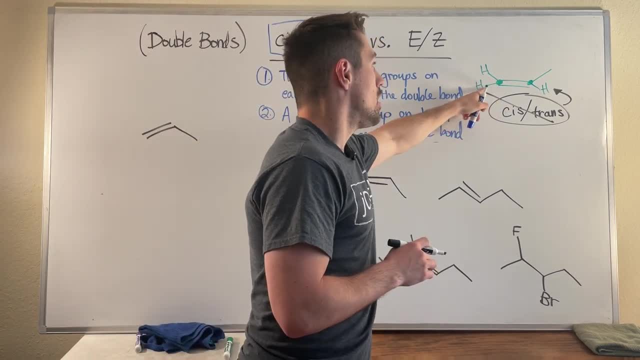 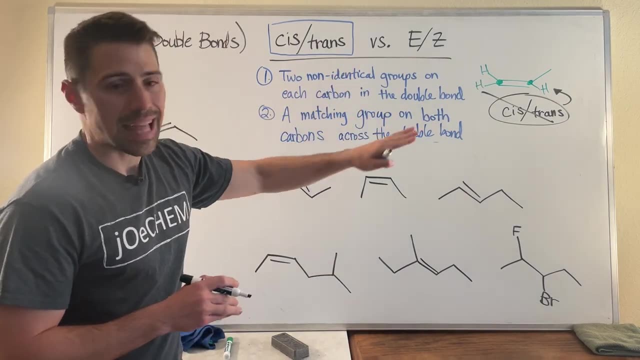 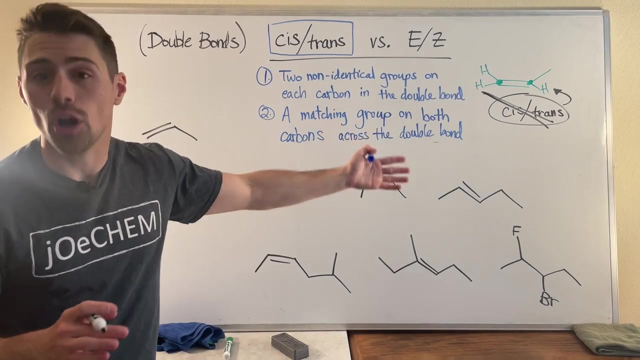 looking at here. But if you look at this carbon right here, it has two hydrogens attached to it. Those are identical groups. So once you see something like that, you can go ahead and just say: I cannot label this double bond as being cis or trans, So you just can't call it either, or 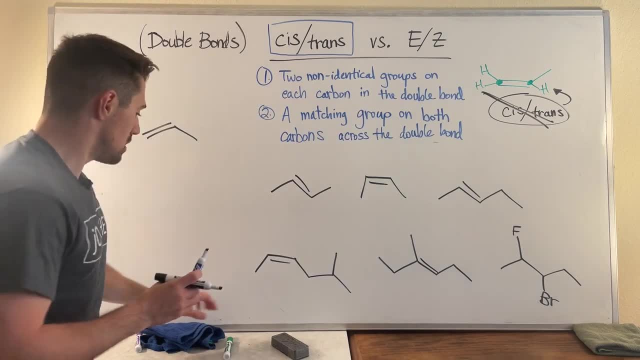 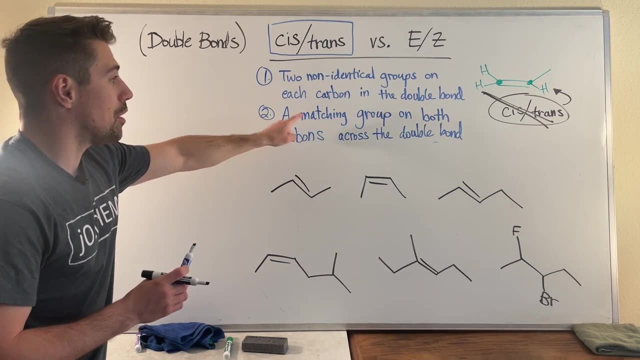 But let's just say you do have criteria one. then you look at number two and you say to yourself: now, if I look at both of the carbons again, does a group on both sides of the double bond match? Here's what I mean by that. If we 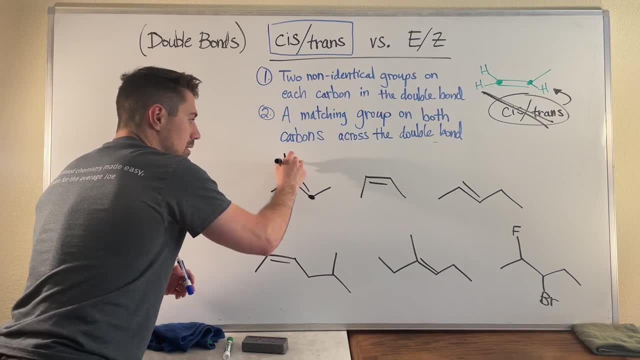 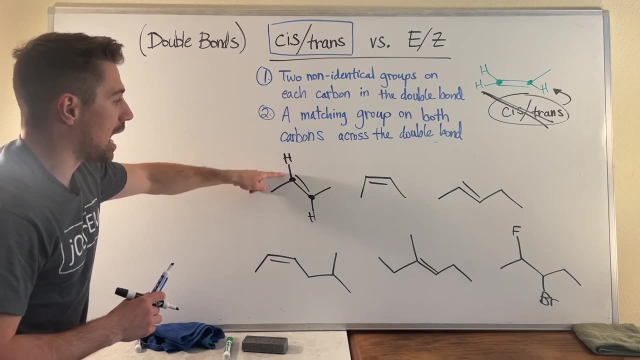 look at this structure right here. let me just list out all the groups attached. Looking at this point, number one: this carbon right here has a CH3 and a hydrogen, So these are non-identical. That's good. If I look on the right-hand side, hydrogen and CH3,. 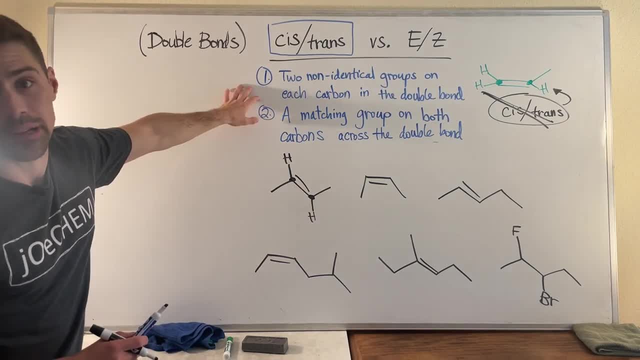 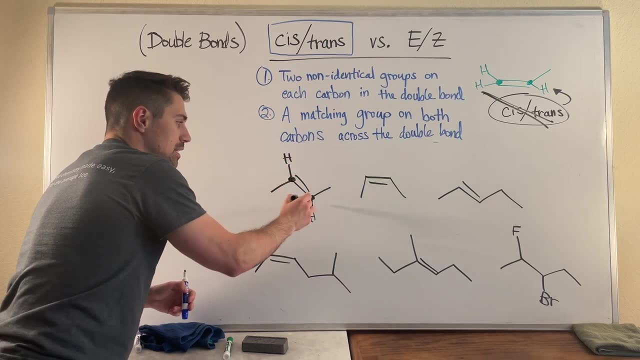 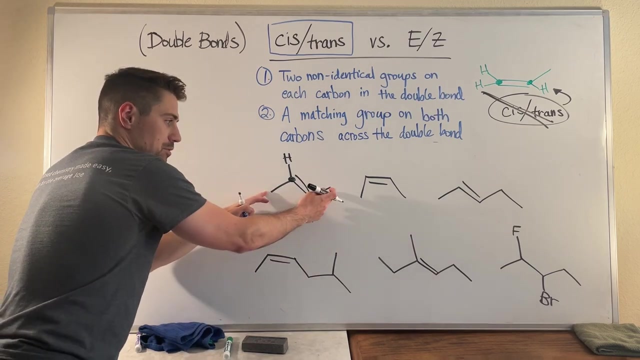 also good. So we've satisfied criteria. point number one. Now for two. we actually have two of these, but you see how there's a hydrogen on this side of the double bond and this side of the double bond. That's what I mean by a matching group. So, and again, we have two methyls here. 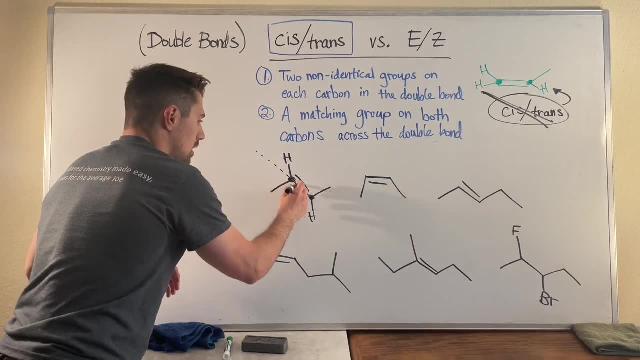 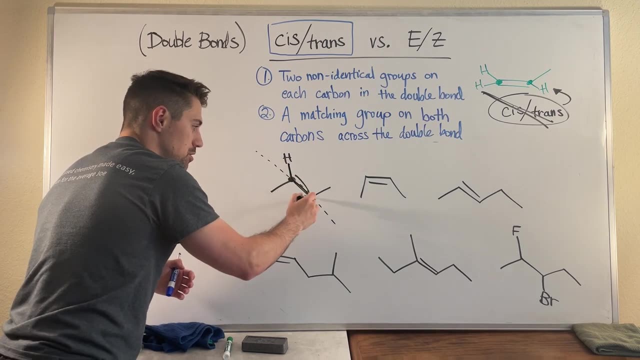 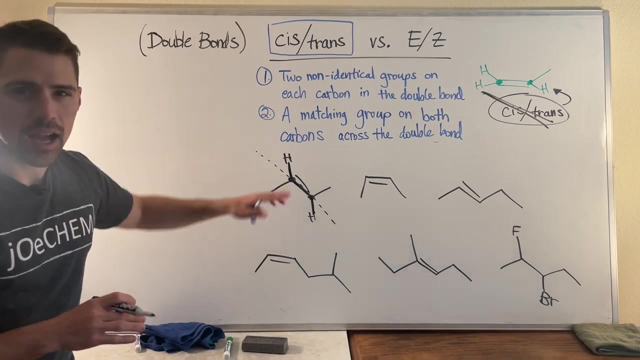 so you can use either or. but if you draw a dotted line across your double bond, go from one of the matching- the one of the atoms in the matching group or you know substituents- to the other. Once you've traced that line, look to see if you've crossed the dotted line or not. If you've, 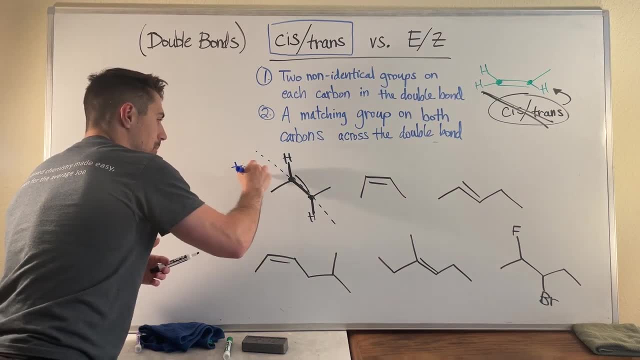 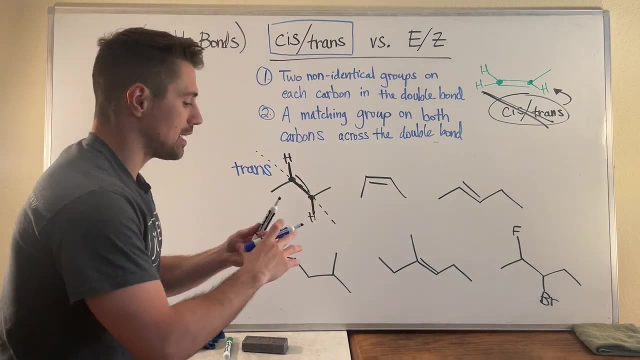 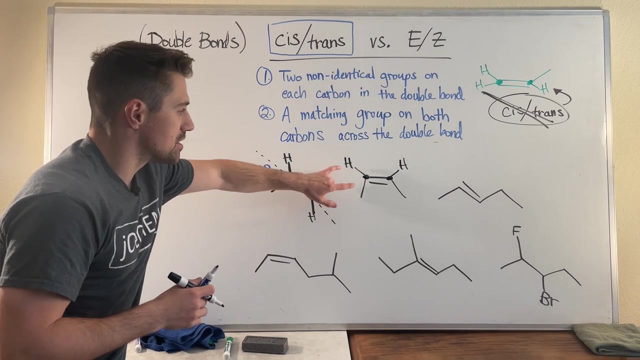 crossed it, that means you have a trans double bond. If you don't cross it, then you have a cis double bond. To show you what that looks like, let's look at this example right here. What you can see is, if we list out the hydrogens here on one side of the double bond, 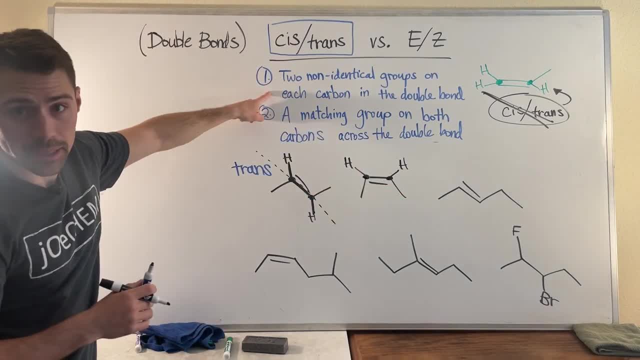 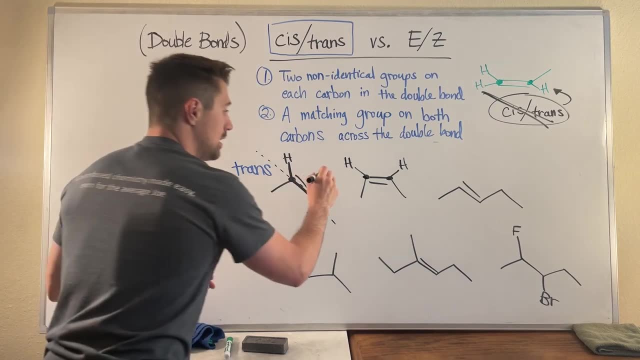 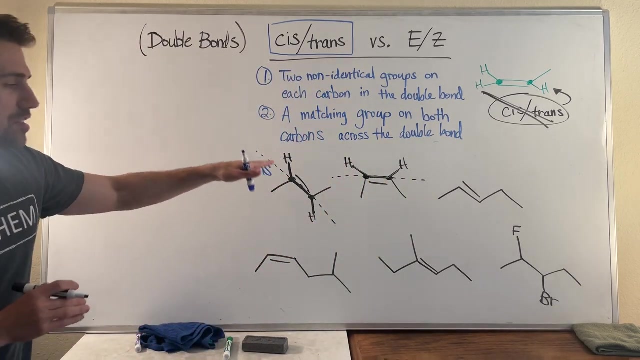 these do not match and these do not match. So we're good up here. You can see we have two hydrogens and two methyl groups, Either one you want to trace. If you draw your dotted line, let's just go from hydrogen to hydrogen. You can see I never crossed. 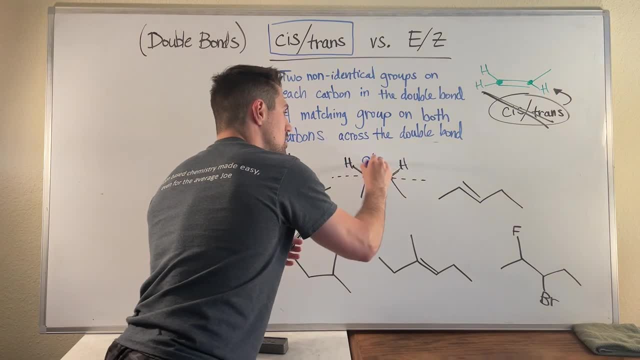 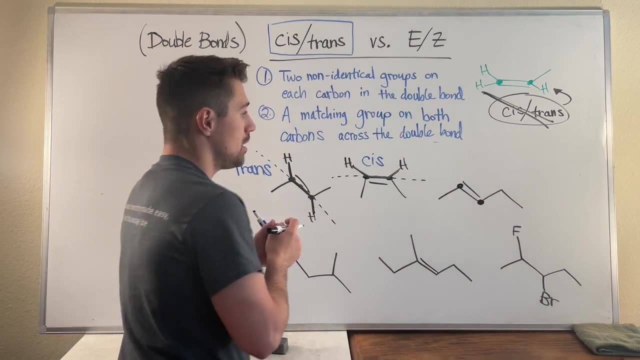 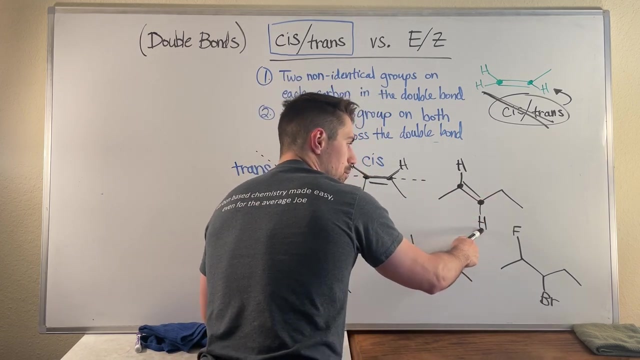 the dotted line. So that means I have a cis double bond. Now let's keep going. If I use this structure right here, you can see all right, on this side of the double bond these do not match. And on this side of the double bond. 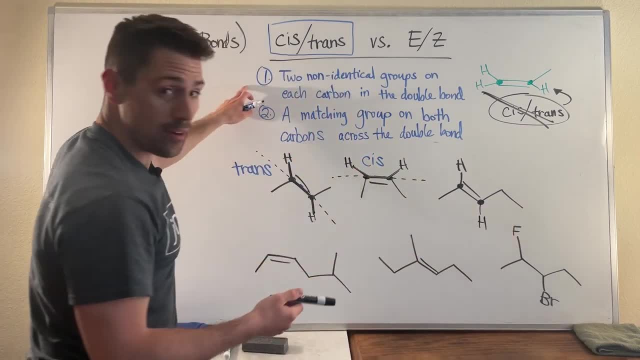 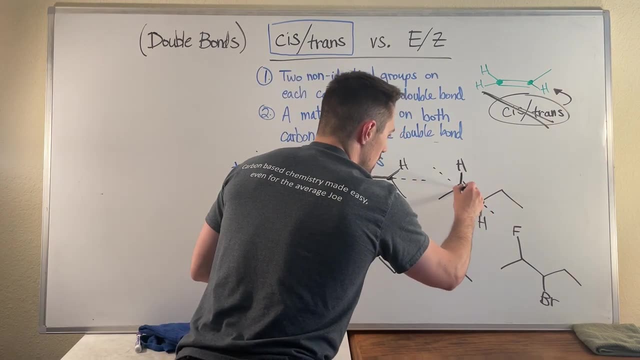 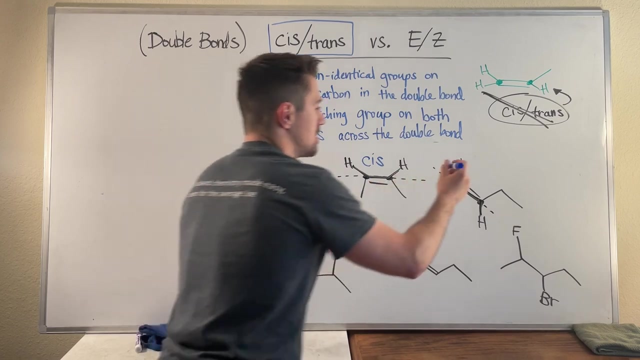 I have an ethyl group and a hydrogen, So we're good on one And for two. you can see, I can just go from hydrogen to hydrogen, because the methyl and the ethyl do not match but the hydrogens do, And you can see, in doing that I crossed the dotted line. So this is a trans double bond. 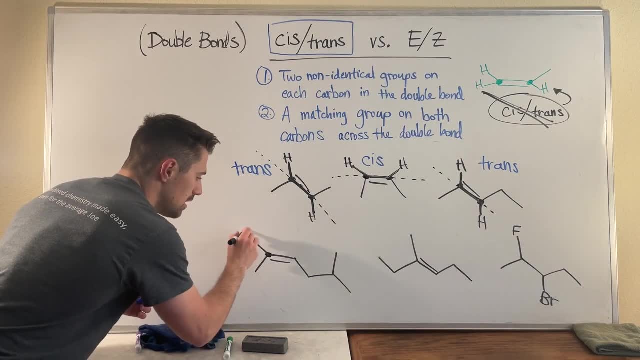 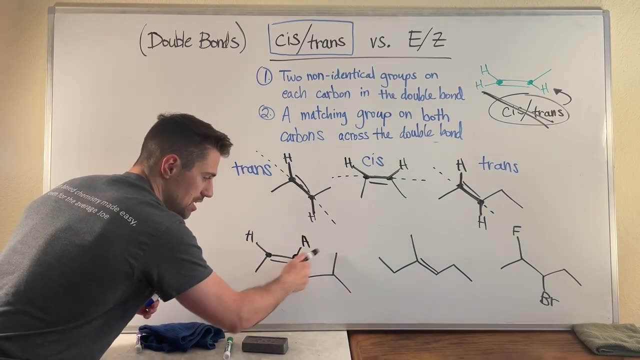 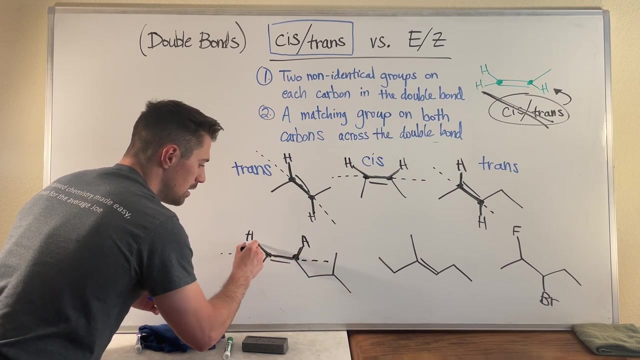 We'll keep on rolling. Over here you can see these two do not match the methyl and the hydrogen. And over here you can see this hydrogen does not match the substituent. down here, If I draw my dotted line, I can go from hydrogen to hydrogen. I never crossed the dotted line. 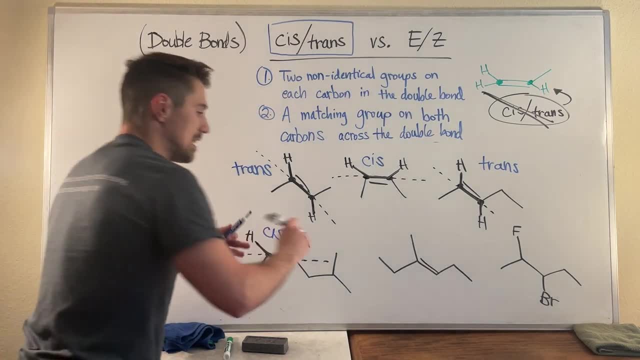 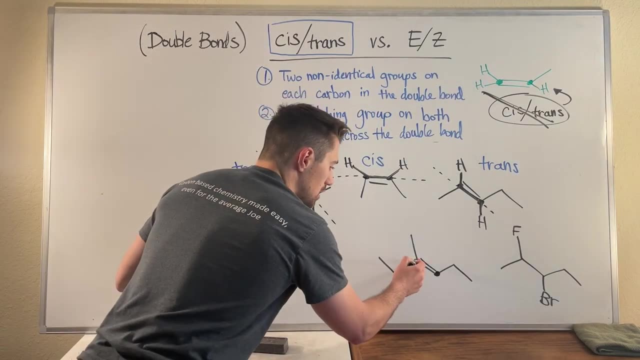 So that is cis. This one's a bit interesting, which is why I like it, But nothing changes in terms of what we know to be true. If I look at this side of the double bond, I have a hydrogen and I have an ethyl, So these do not match. 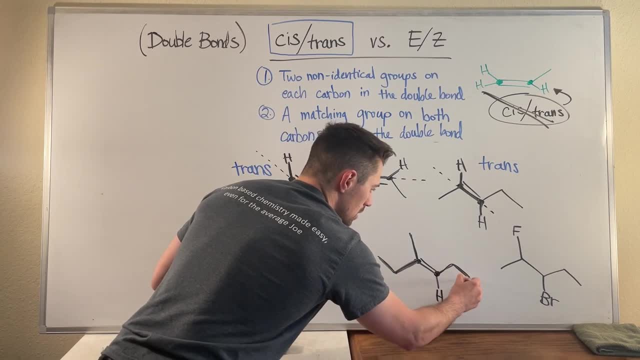 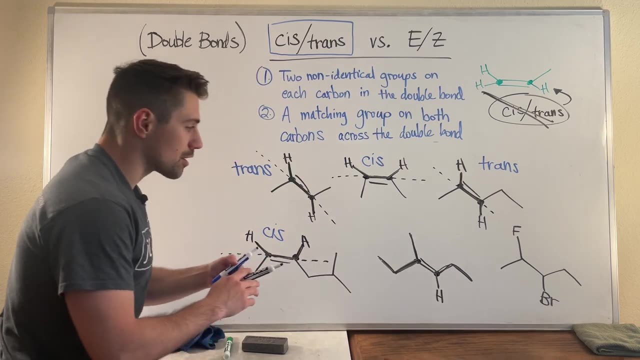 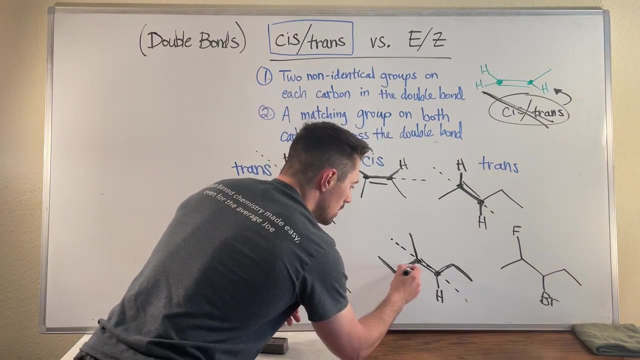 Over here I have a hydrogen and an ethyl, So we satisfy point number one because nothing matches on each individual side. However, if I'm trying to find my matching group across the double bond, I can go from ethyl to ethyl. Okay, A bit weird, but ethyl to ethyl. You can see I crossed my. 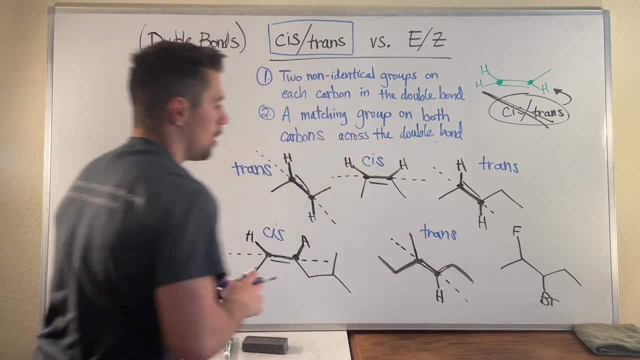 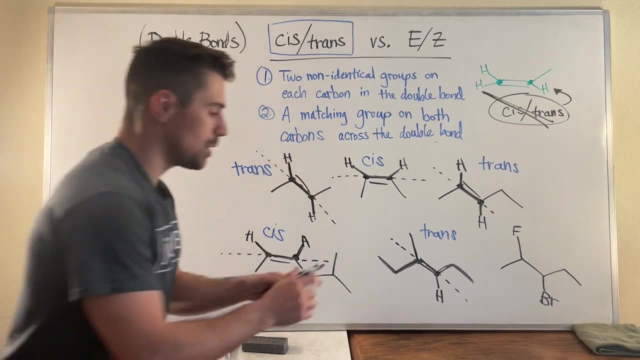 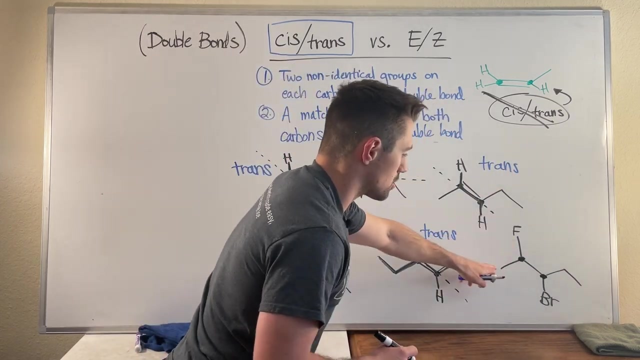 dotted line and this is trans. Okay, So everything I've shown you up to this point can work with cis-trans terminology. However, if we see a situation over here, while our first criteria point works right, The fluorine does not match the methyl. 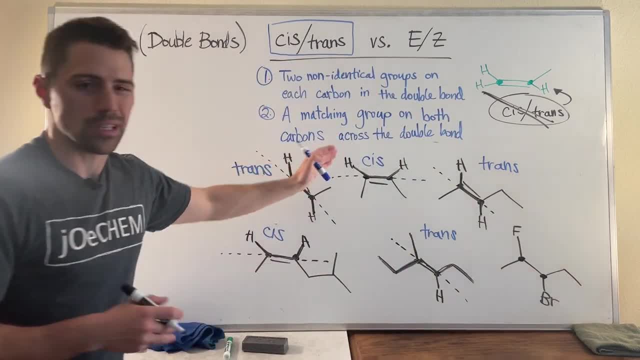 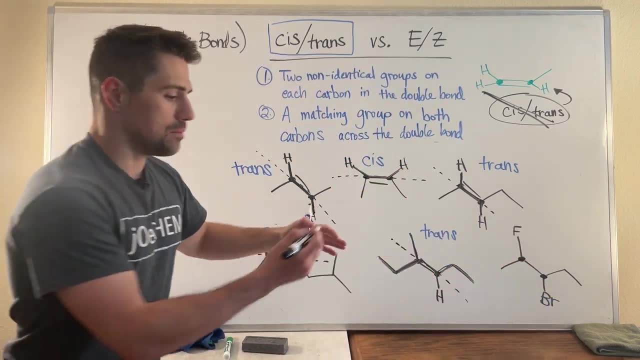 the ethyl does not match the bromine. We break down at point two because nothing matches across the double bond. I don't know where to start and where to trace to. This should be a double bond. I'm sorry, Whoops Forgot that the whole time. When you have a situation like that, that means you. 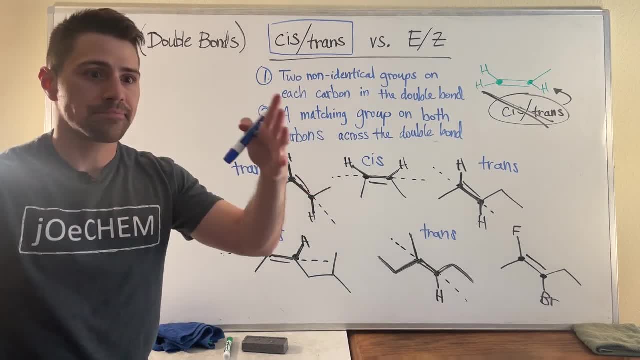 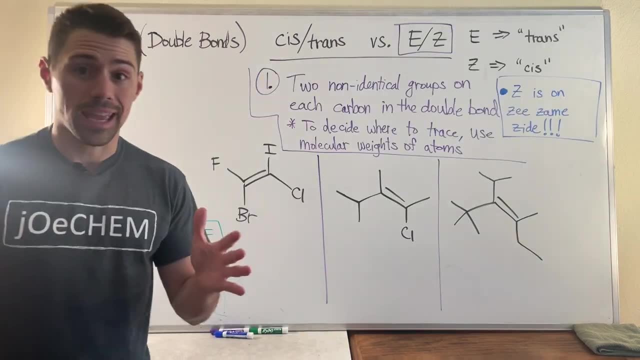 can't use cis-trans terminology. We can't use cis-trans terminology because it's not the same. You need something a little bit more general, And that is where ENZ terminology comes in. So let me erase this. We'll be right back. Okay, gang. Now I want to move on from. 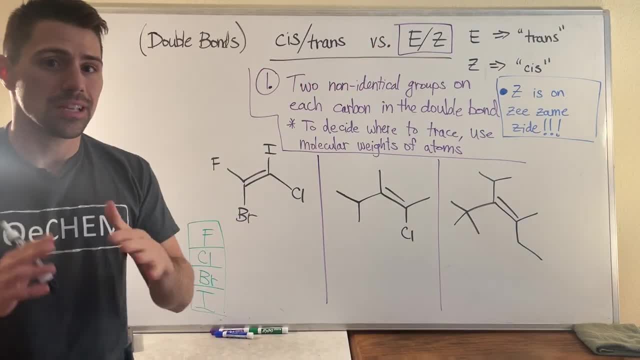 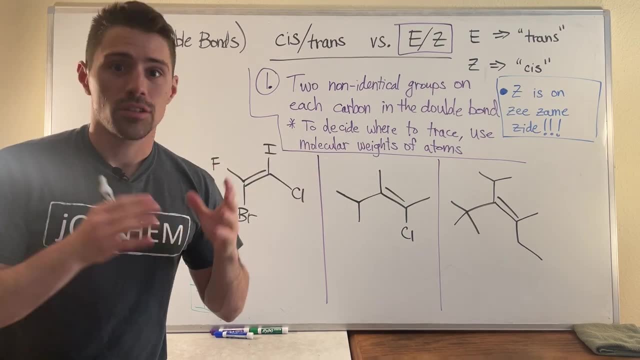 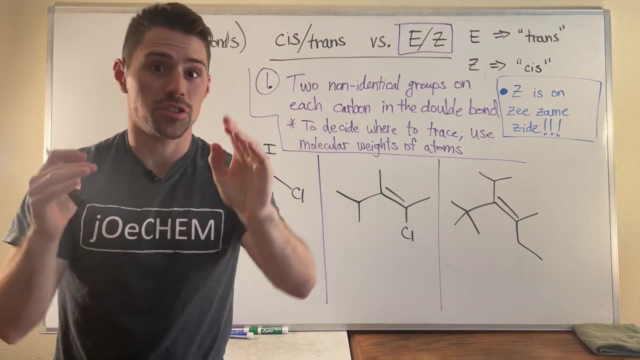 cis-trans to ENZ. The important thing to note is that if you are using ENZ- or, sorry, cis-trans terminology- you are able to use ENZ terminology. Think of ENZ as like a big umbrella, and inside that umbrella is the cis-trans terminology, So you can always use ENZ. 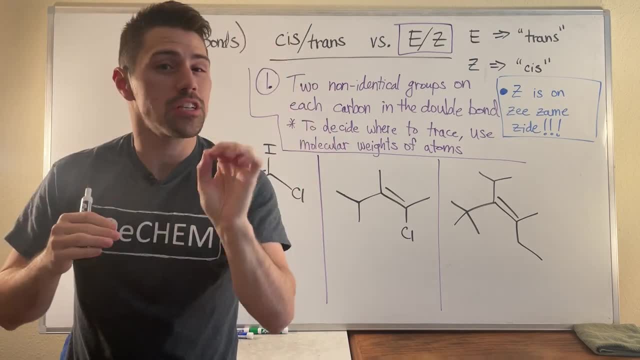 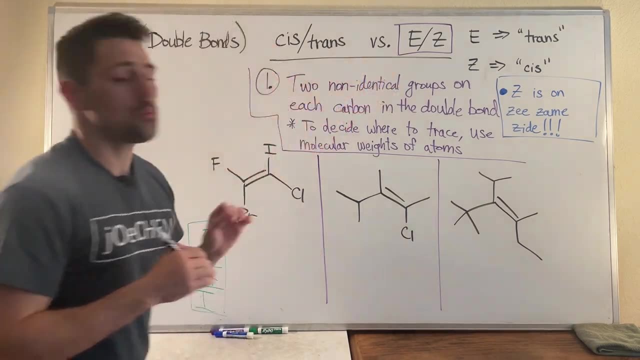 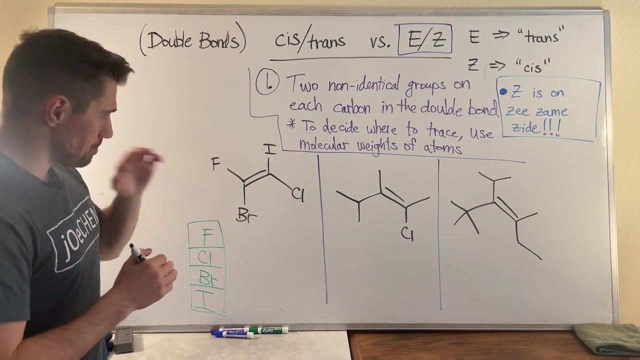 and it's more like if your situation is specific enough, you can use cis and trans. Here's what I mean. You only have one point of criteria. when you can label a double bond as E or Z, you know, and that point of criteria is something we're familiar with- You just need to have two non. 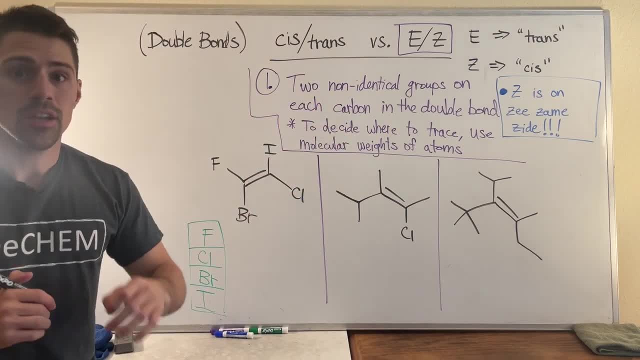 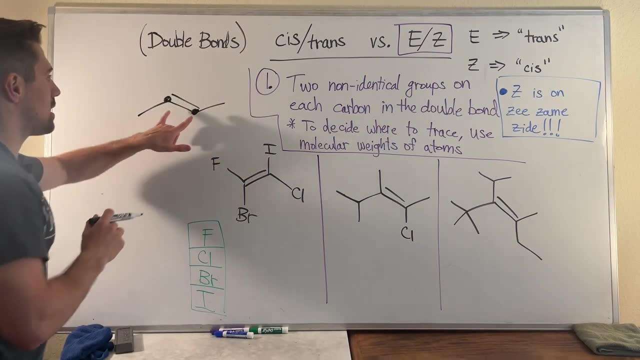 identical groups on each carbon in the double bond. What we mean by that is, if you look at both sides of the double bond, you're going to have two non identical groups on each carbon in the double bond. You just need to make sure that when you look at each carbon, just like we did, 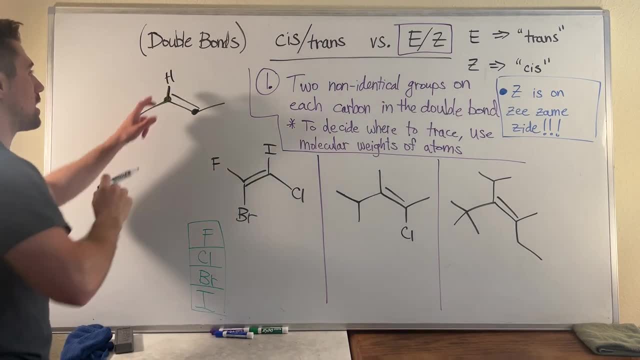 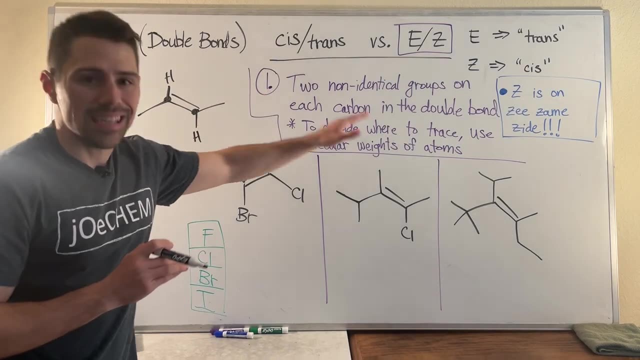 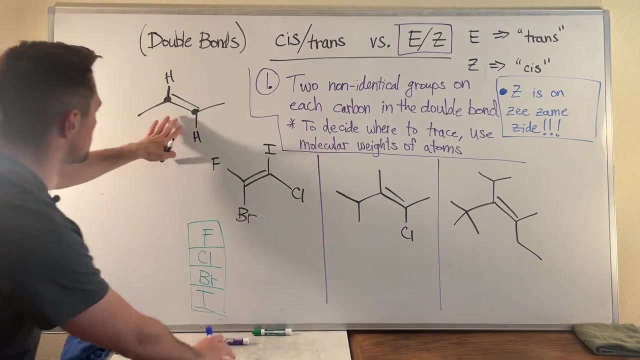 previously. these two groups cannot be the same. So right now we have a hydrogen and a CH3 and a hydrogen and a CH3.. That is it. Now, the way you go about assigning ENZ is slightly different. Let's take this: If we were doing okay, there we go. If we were doing a cis and trans here. 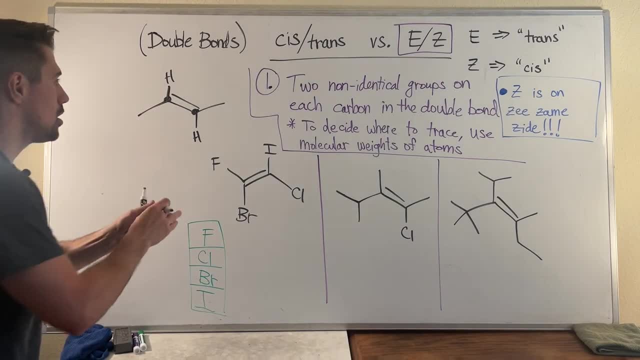 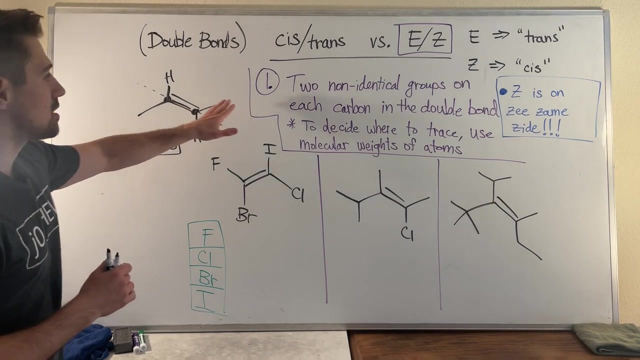 we would just take one of the matching pairs and trace it right So we could go from hydrogen to hydrogen and we would know we're crossing the imaginary double dotted line. So this would be trans. To find out what would this would be in ENZ terminology: you look on both sides of the 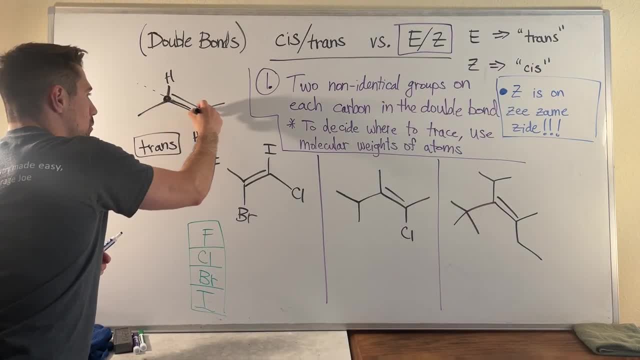 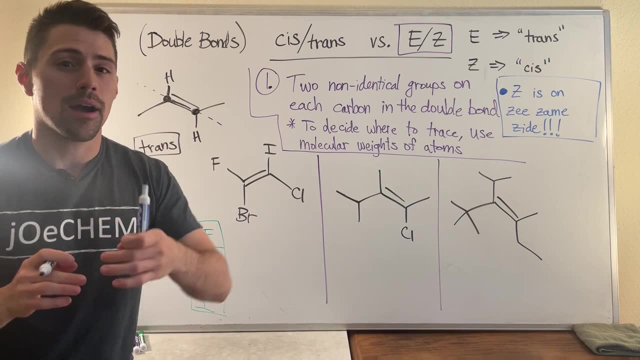 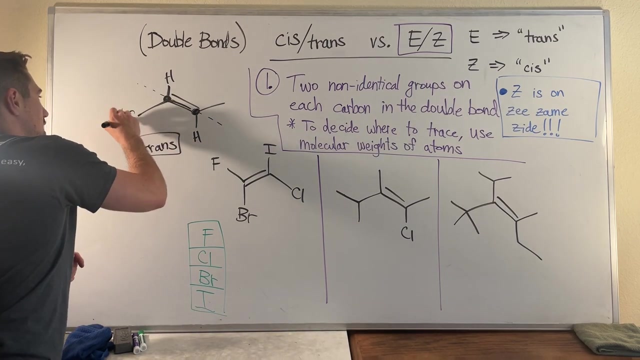 double bond and for each carbon in that double bond you look at what we're going to call the highest priority group, And by highest priority we're talking about what is the heaviest atom by molecular weight. So if we take a look here, I know that I have a CH3 over here and a CH3. 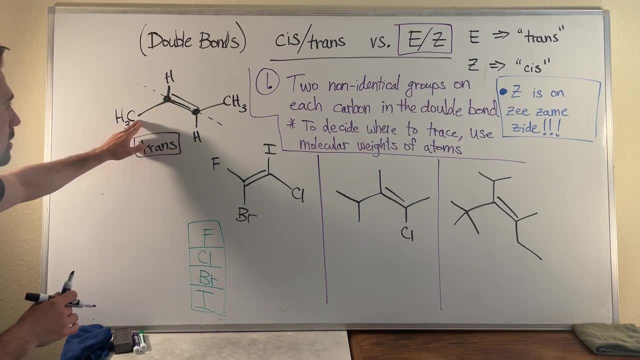 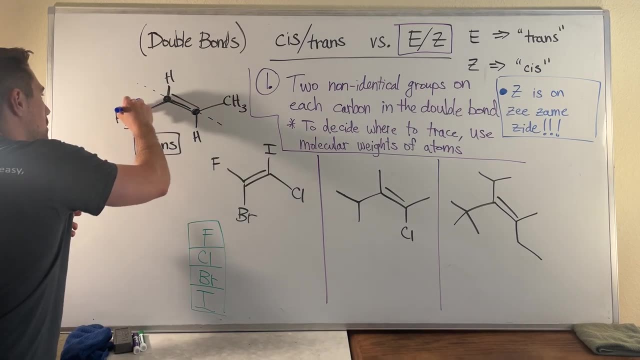 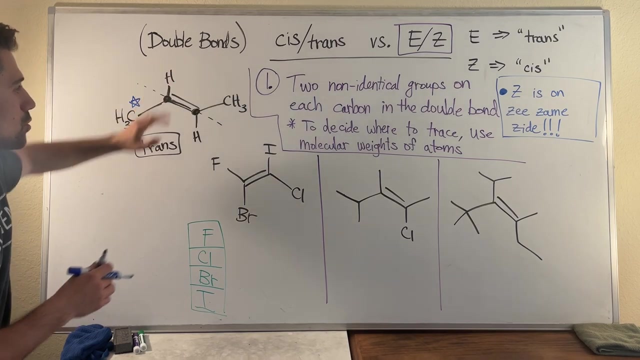 over here, Directly off the double bond. I have a carbon and I have a hydrogen. Carbon is much heavier than hydrogen, So this is my higher priority group on this side of the double bond. So I'll put a star there. On this same side of the double bond, same story: This carbon is heavier. 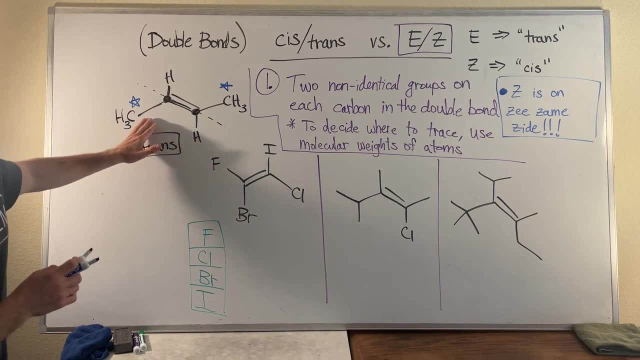 than this hydrogen. You then trace from your hydrogen to this hydrogen. You then trace from your highest priority on one side to the other side. So again this happens to be carbon to CH3 to CH3.. So you can see, I've crossed my dotted line. Now the parallels you can draw between cis: 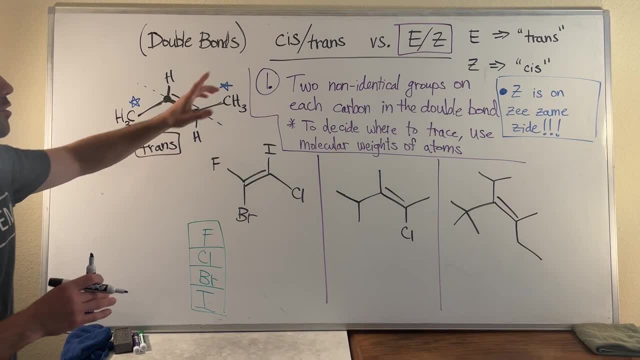 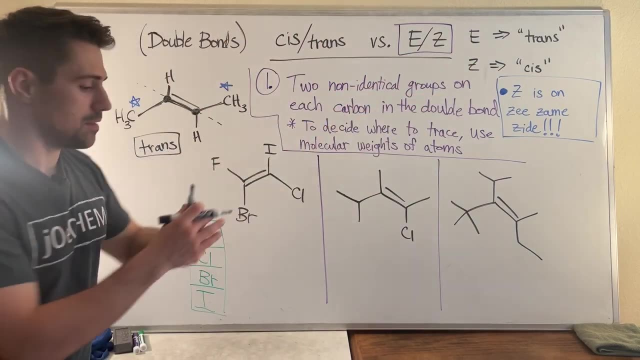 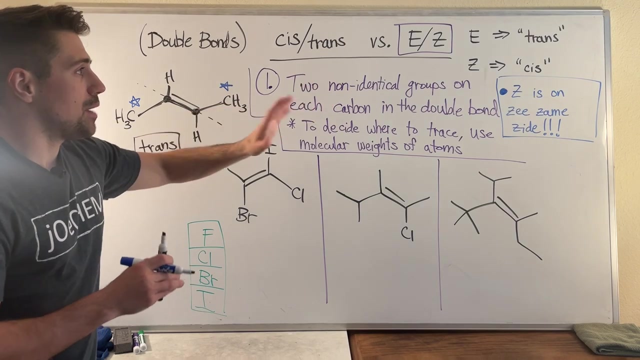 trans, and E and Z is that if you are crossing the double bond, the dotted line, rather, you are E. E is like your trans equivalent. So this is E, The way I usually like to remember it. Z- if you end up on the same side of your dotted line, that means that Z is on the same side. 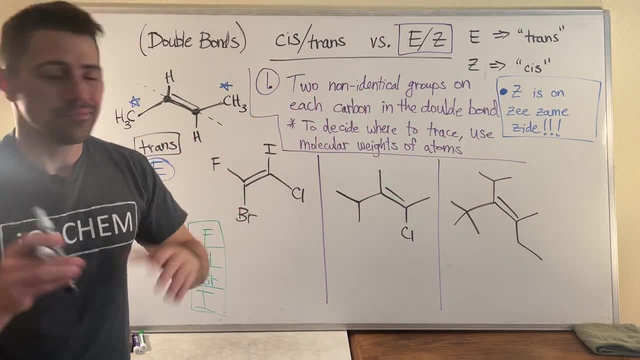 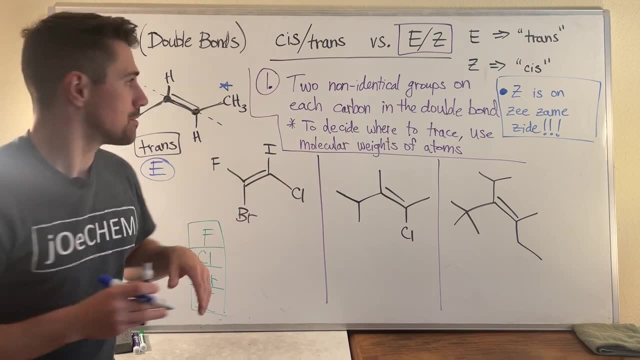 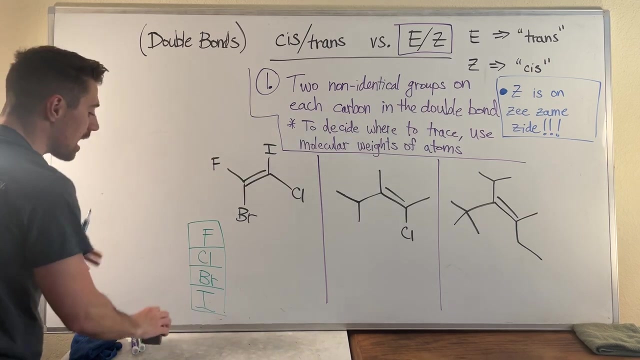 So Z is cis and E is trans. So that's how I kind of remember it. Z has that nice like, so Z is the same as cis, E is trans. So that is the only thing you need to do for this And you'll see how we- if sometimes you- end up having ties. 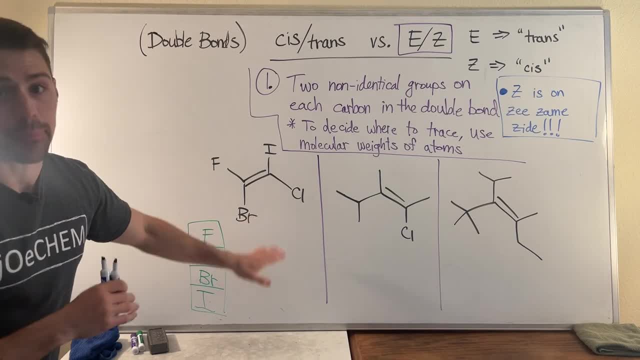 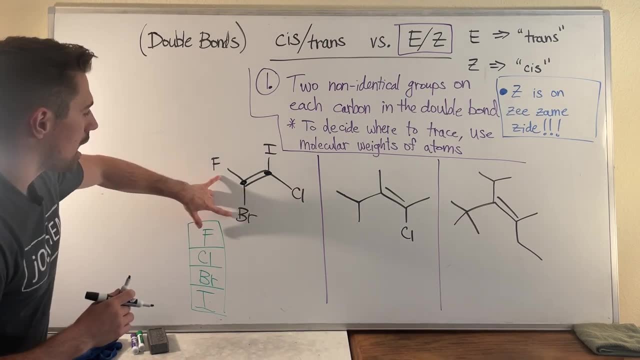 show you how to break ties. So let's take this original example that brought us here in the first place. If we take a look at this structure, you can see that on each side the fluorine does not match the bromine, The iodine does not match the chlorine, So we can use E and Z terminology here. 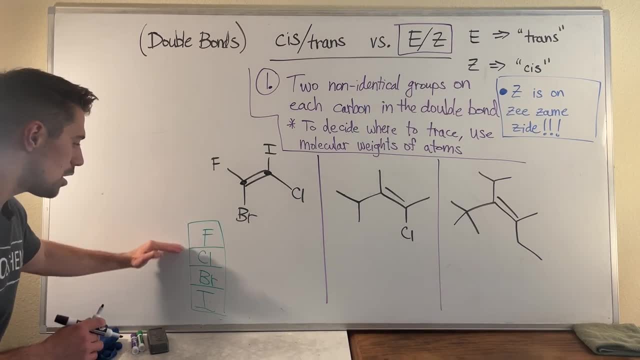 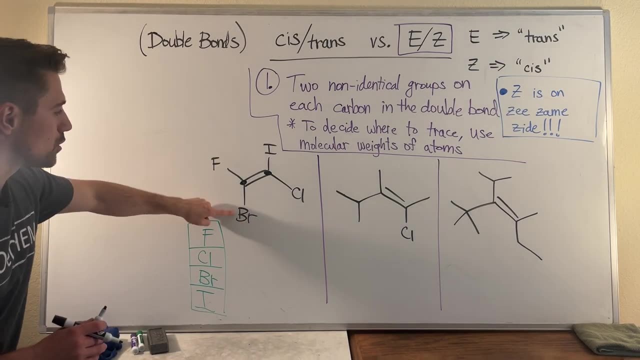 I took a little snippet of the periodic table here, because as you go down the periodic table molecular weight goes up, right. So on this side of the periodic table we're looking at fluorine. you know this. sorry, this side of the double bond, rather. 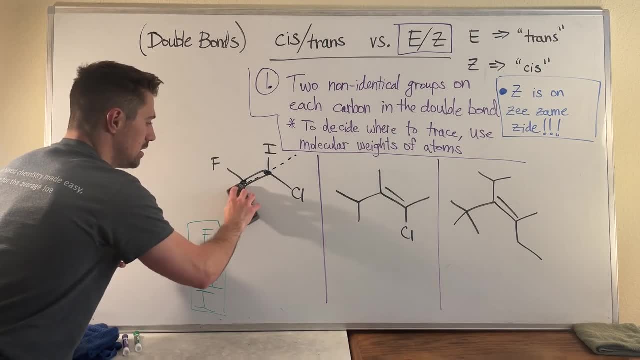 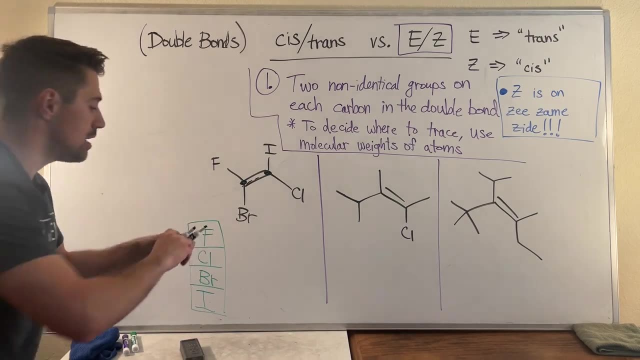 we have fluorine and bromine. Speaker 1. Actually, let me wait to draw the dotted line. Sometimes it gets a bit confusing. So fluorine is not as heavy as bromine. Bromine is the heavier molecule. As a result, it is higher priority than fluorine. 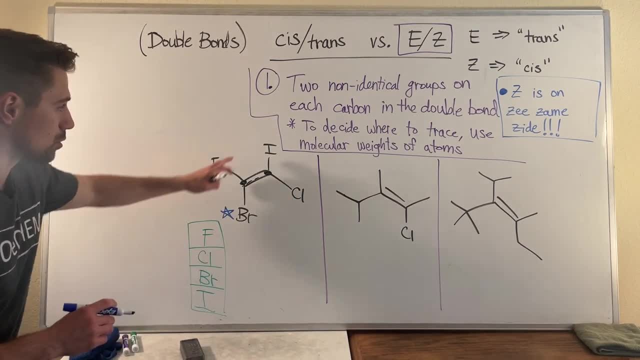 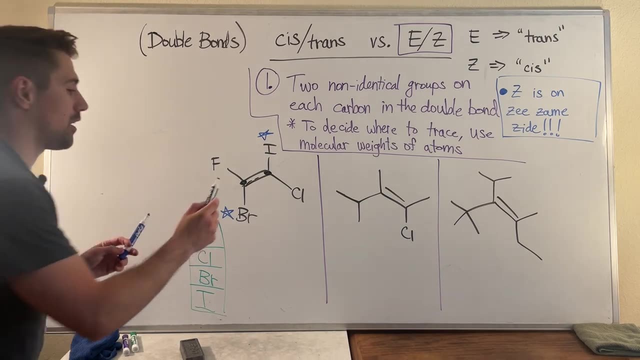 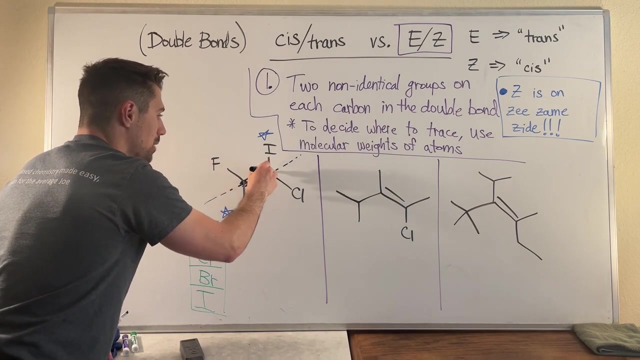 So we've got this side figured out. Now, on this side, we have iodine and chlorine. Iodine is lower, so it is higher priority relative to chlorine. Once you've identified your priorities, draw your dotted line, Go from highest priority on one side to the highest priority on the other side. 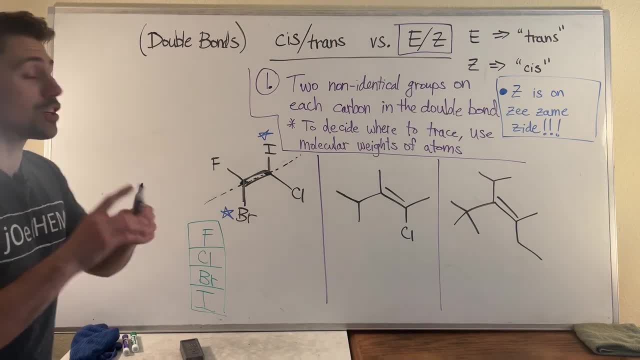 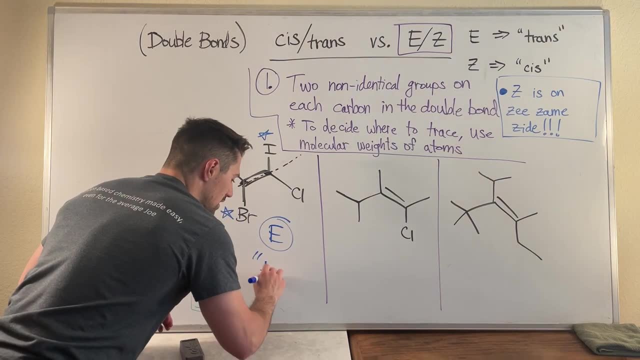 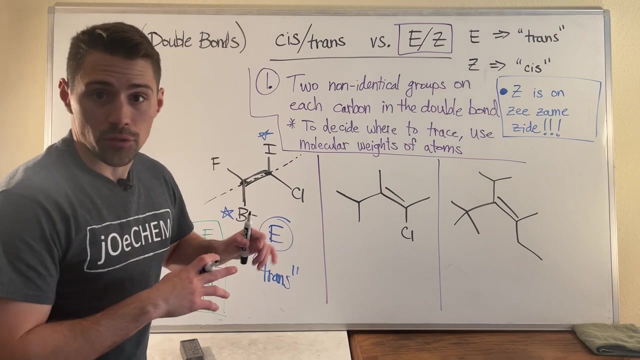 You can see we are crossing the dotted line, so we are not on the same side. So it's not Z, we are E, Or you can think of this as trans, even though that is not the proper use of the term. Let's look at this double bond over here. 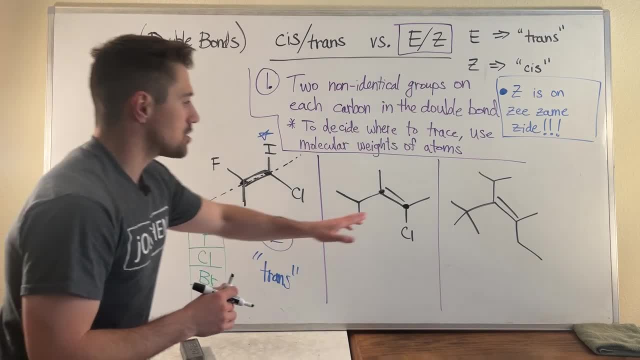 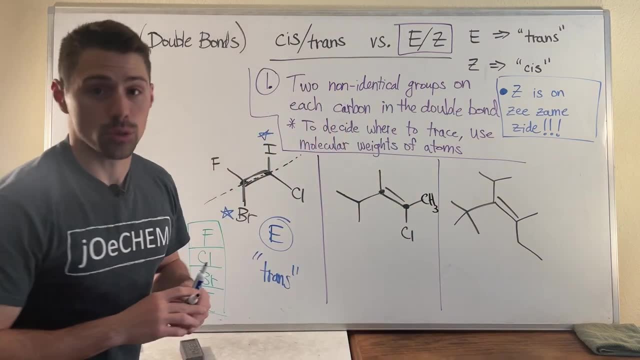 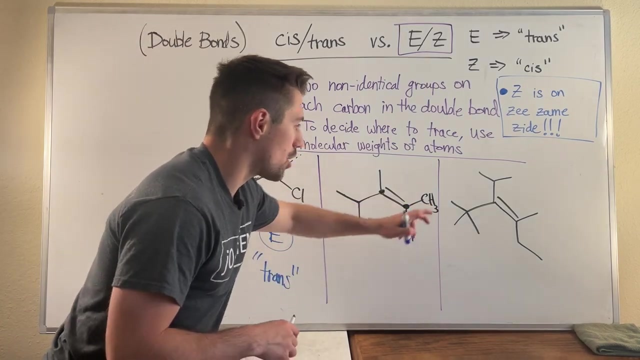 This is where things get a bit more interesting. Now let's go on the right-hand side. first, I would be comparing a CH3 and a chlorine, So you always want to consider the atom directly attached to the double bond. We have a chlorine versus a carbon. 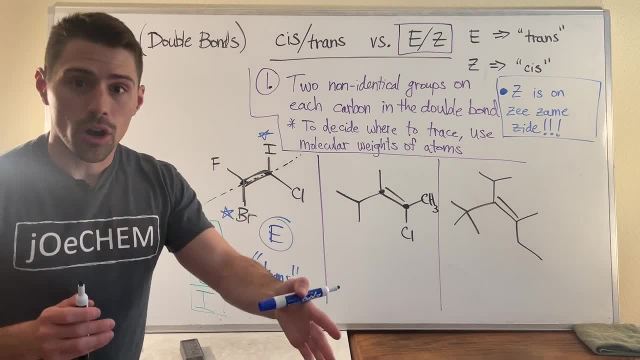 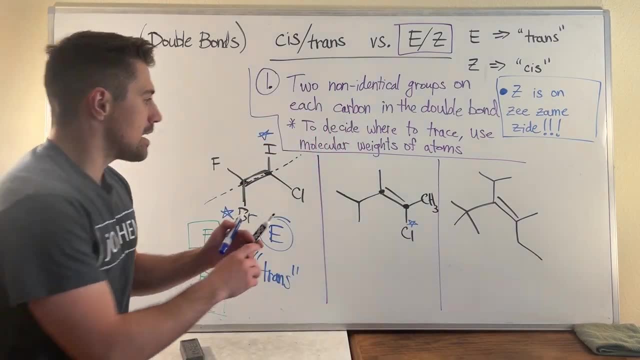 If you look at a periodic table, chlorine is much heavier than carbon in terms of molecular weight, So chlorine is our higher priority group here. Now, when I look at the other side of this double bond here, I have something interesting. So I have a CH3.. 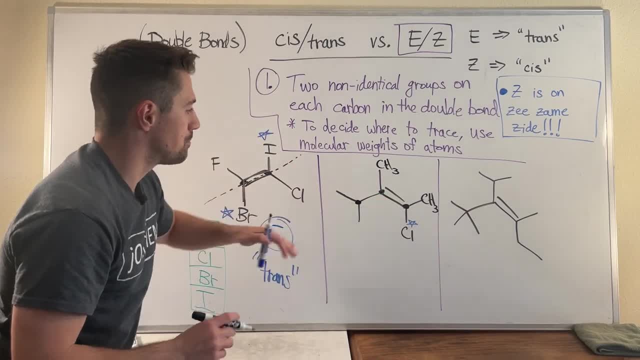 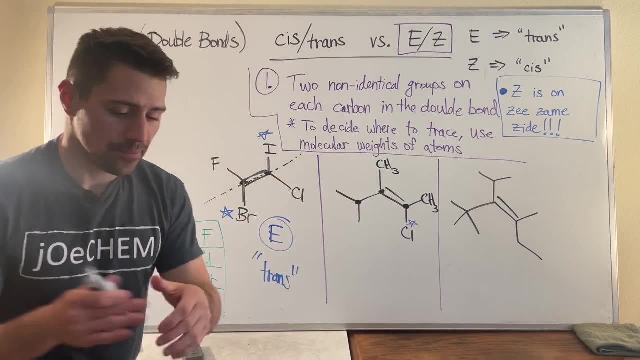 And then I have this group right here, this isopropyl group. Now, when I just consider the first atom attached, I have a carbon versus a carbon. So we have a tie. Here's how you break ties. I like to draw this out. 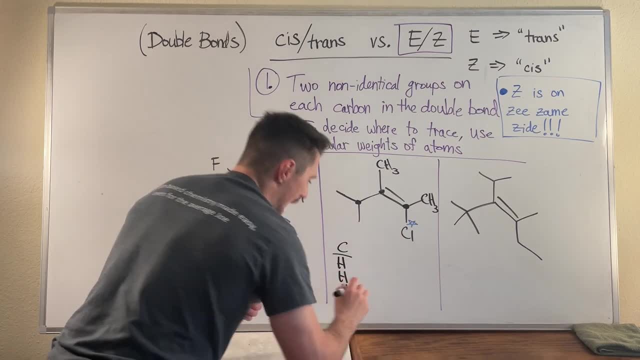 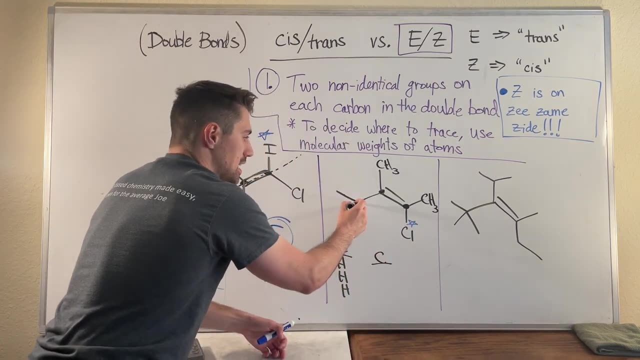 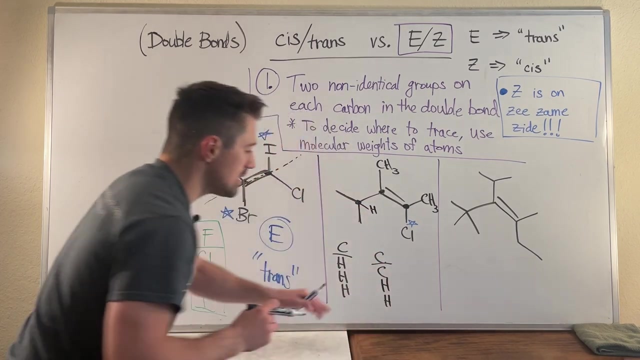 So I have a carbon and then list out everything that's attached to it. HHH, Over here I have this carbon and it is attached to a carbon. a carbon and one hydrogen. List them out from the heaviest things that it's oh, two Cs. 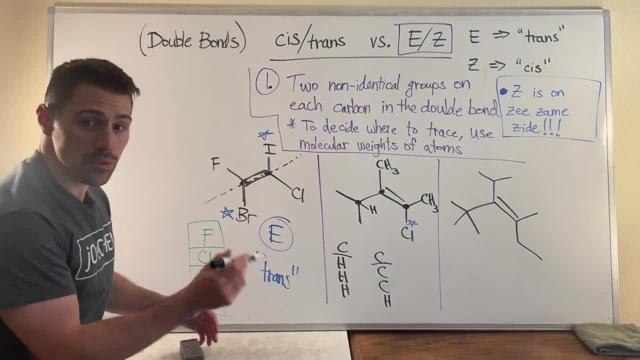 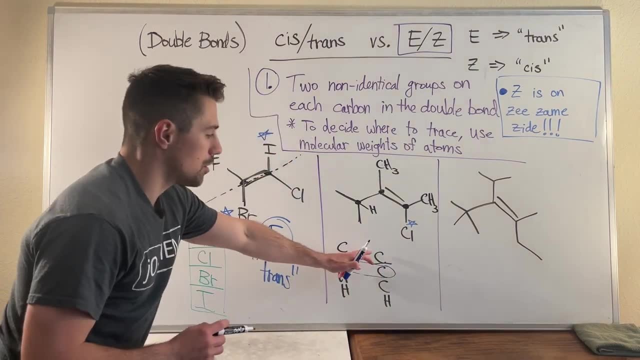 List out the heaviest things first, because what you can do then is you can say, okay, this carbon is here, this carbon is here, and then go until you have a first point of difference. Ah, okay, This carbon. you know we had a tie, but it's attached to heavier things than this is. 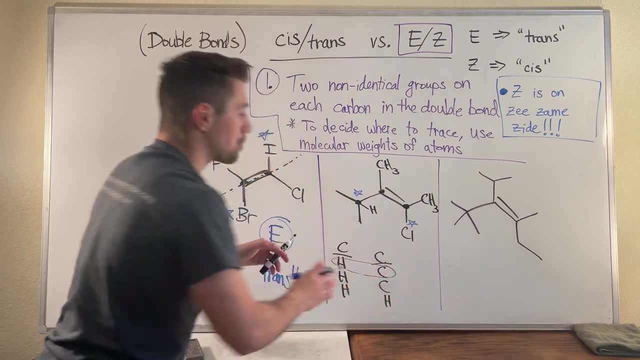 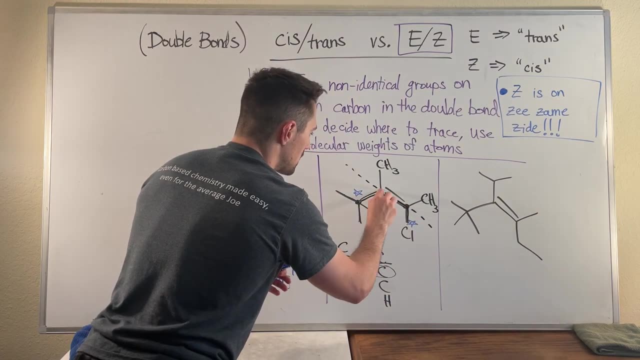 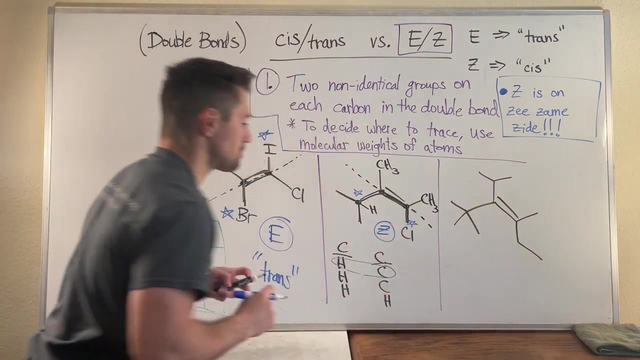 So that means that this is your higher priority group. Then you can draw your dotted line. Okay, Then you can trace from highest priority to highest priority. You can see, here we end up on ze same side. So this is a Z double bond. 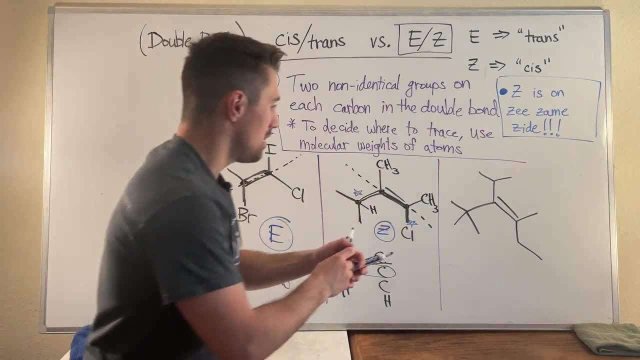 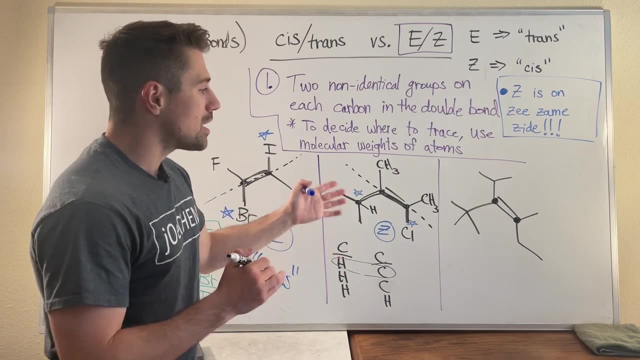 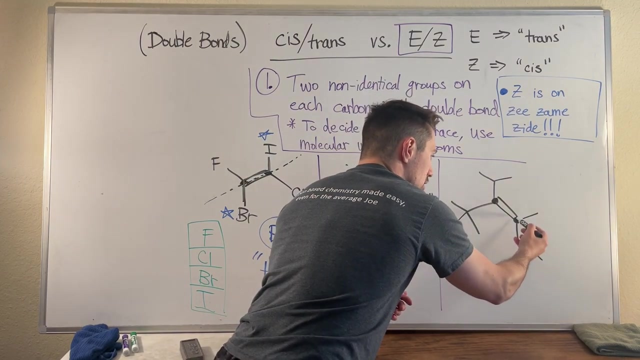 Last but not least, I wanted to make things even more complicated. You can see, clearly we have non-identical groups on both sides, And what I try to do here is basically cause a bunch of ties. So on this side of the double bond, we have an ethyl group versus a methyl group. 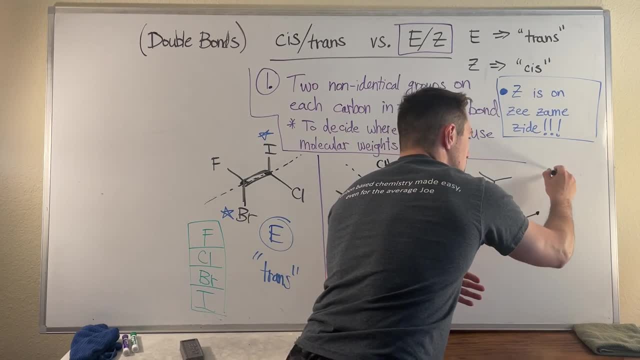 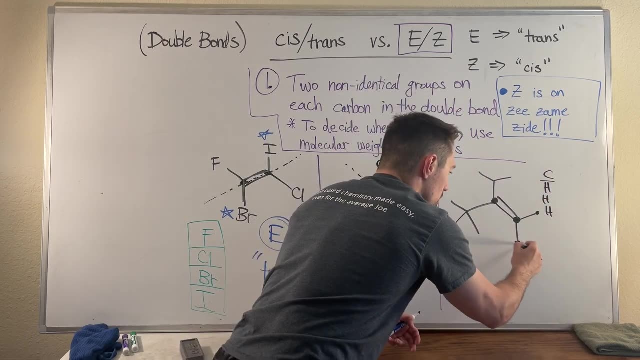 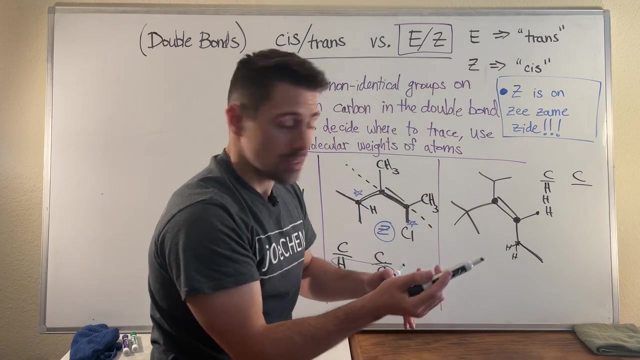 So to do the tiebreaker right here, this is C attached to three hydrogens. So I'll do H, H, H And over here. this carbon, which I'll draw over here, is attached to one carbon and two hydrogens. 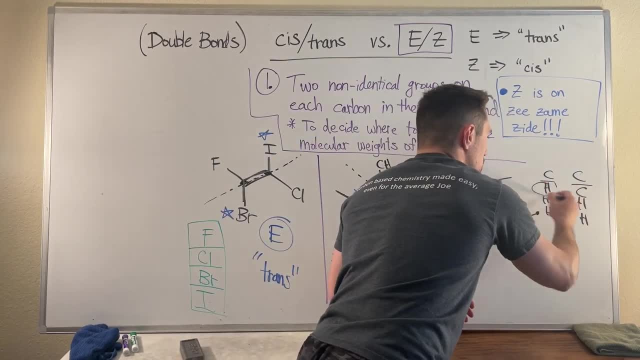 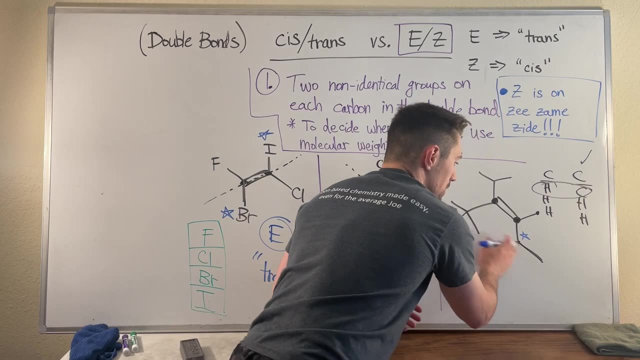 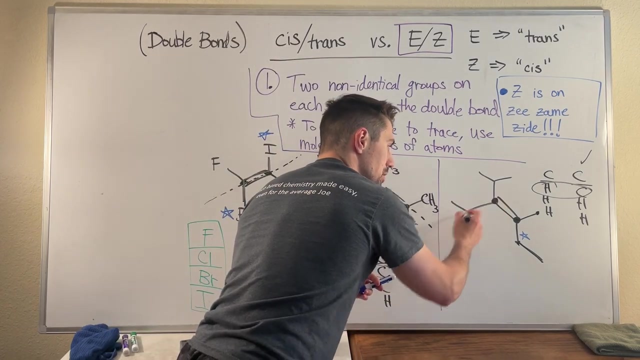 So it is C, H, H. First point of difference is here. This is the higher priority group. I'll put a little star right next to the ethyl group And you can see we'll employ the same strategy. up here, This group, right here, this T-butyl group, this carbon is attached to a carbon. a carbon and a carbon.